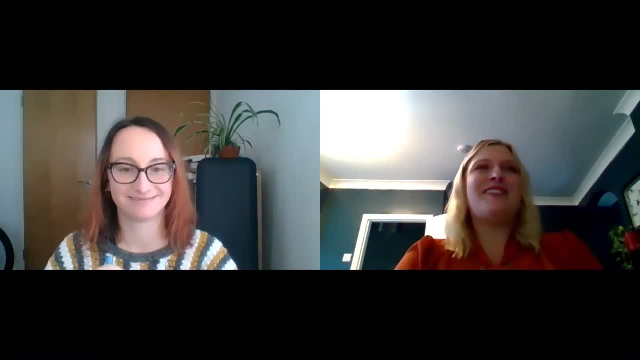 changed past thousands to millions of years. So, Anna, thanks so much for being here. If you have any questions for her, just because we're recording this, we're going to use the Q&A function rather than allowing me to ask them out loud. 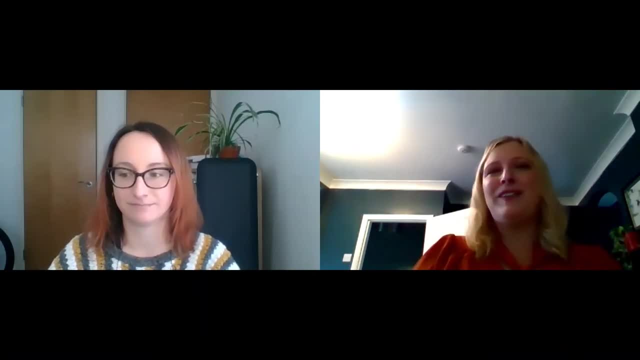 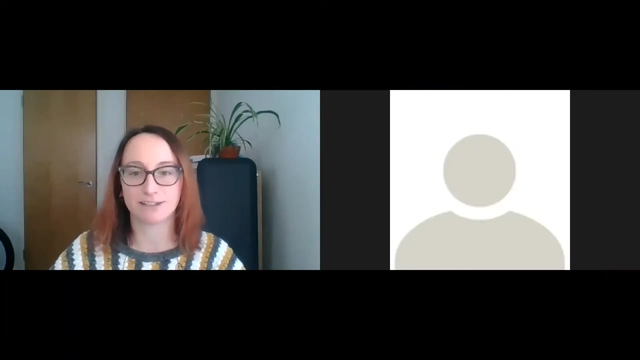 So, please, if you have a question, as she's kind of telling you a bit about herself- please pop it in the Q&A box And we'll spend the rest of the session answering some questions. So, thank you, Anna. please take it away. Thank you very much. I'm going to share my screen with you all. 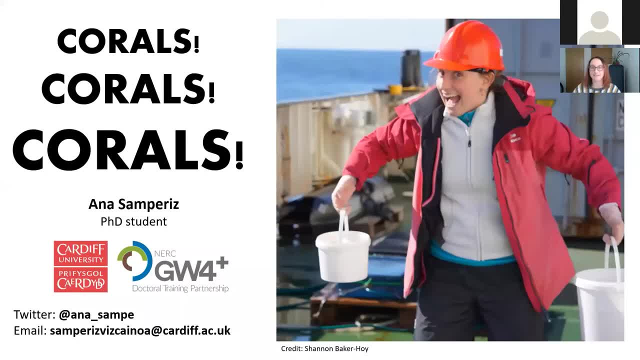 so you can see the slides. I have prepared slides. I think you should be able to see my screen now. Excellent. Well, thank you everyone for being here And thank you for the opportunity to be here talking to you about corals. So my name is Anna. I'm a coral scientist. 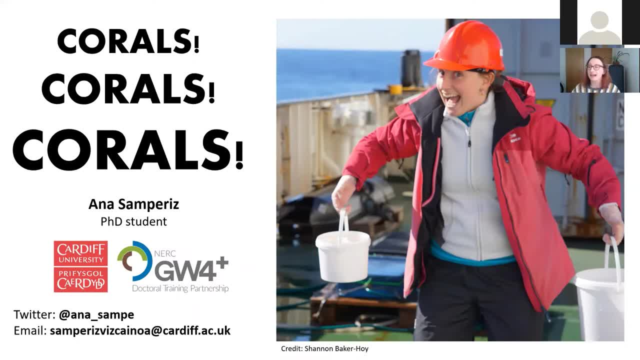 and a PhD student at Cardiff University, And currently I'm working on corals from Fiji. So, in case you haven't noticed, I really, really like corals. Corals are extremely interesting for us And I would like to talk to you about them And hopefully you'll learn a little bit more. 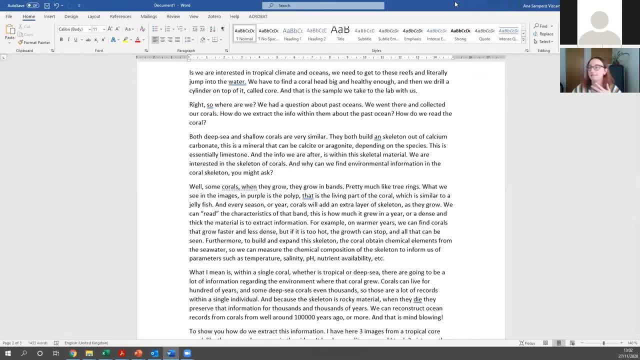 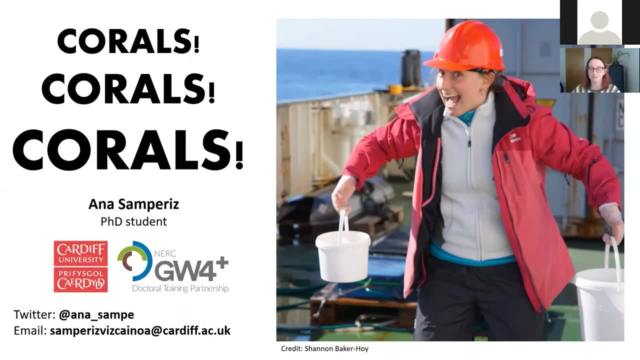 about why they are so interesting, But everything. as we said, a few years ago, I didn't know absolutely anything about corals. I did environmental science for my undergrad in Spain, where I'm from, And back then I had no interest for the sea. I didn't take any course on. 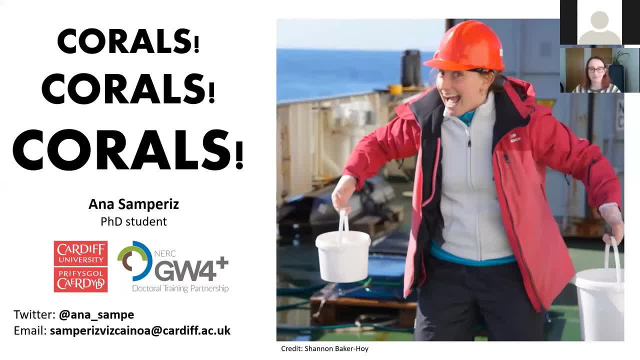 marine science or oceanography, The sea was something that was just just very far away and not appealing whatsoever. So how did I end up as a coral scientist, you might ask? Well, what I was interested in was climate change. what is going on with Earth's climate? 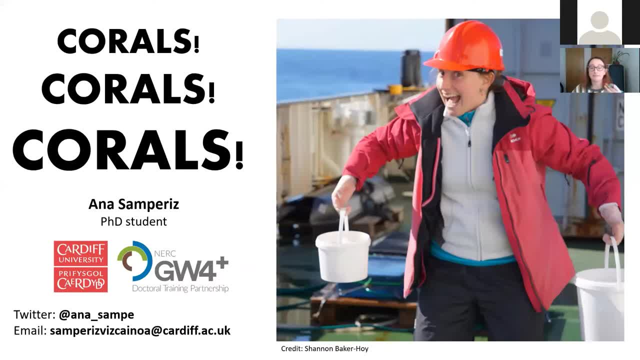 and what is going to happen in the future. These are big questions that are asking ourselves as a society, as we are facing the climate emergency at the moment. So, as it turns out to be able to understand the climate, and what's gonna happen in the future? 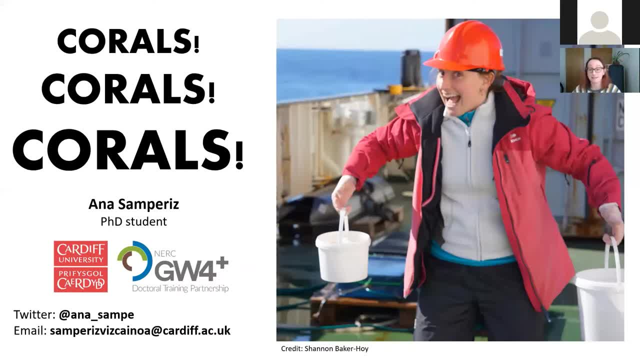 we need to understand how it works And for this we need to look at past climate and how it evolved. That's what we call paleoclimate- the climate of the past. Cool, so we know that I was interested in climate and I went into paleoclimate. 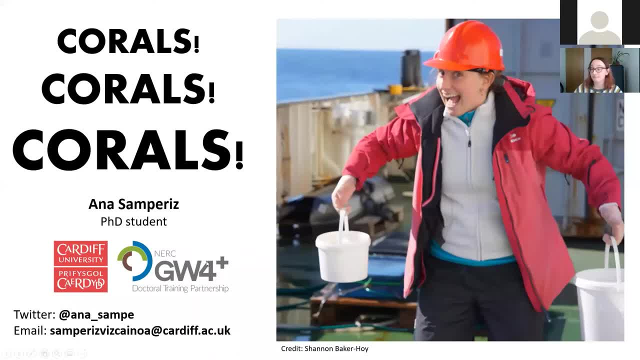 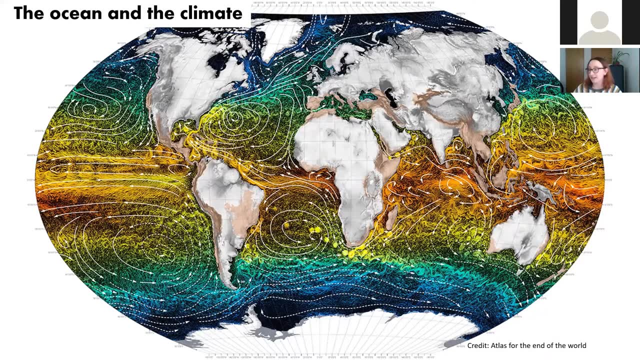 Where do corals come in? Well, in terms of climate dynamics, the oceans play a very important role and they play a key role. They are a major carbon reservoir. They take carbon dioxide from the atmosphere. They are a major heat storage and transport system. 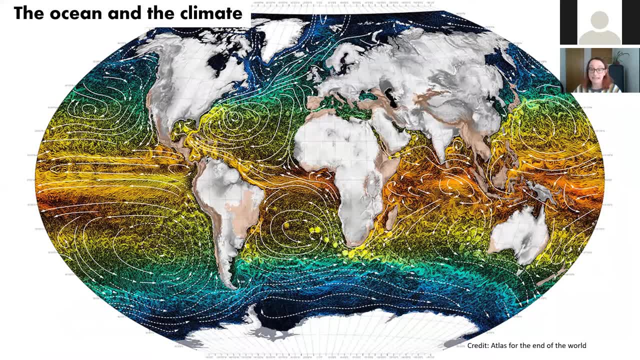 So ocean and climate, they are intimately linked. Clues to the past climate and to the future change can be found in the ocean record. Ocean record: what it is. what do we mean when we talk about ocean record? That's how we find how the ocean was in the past. 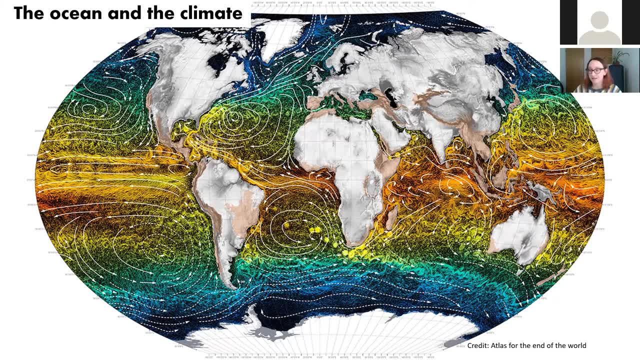 We investigate marine archives. Some archives might be the shells of forums, the shells of bibles or corals, among others. Corals is the archive that I chose. They're called archives because they record the environmental conditions in which they grow and they preserve them. 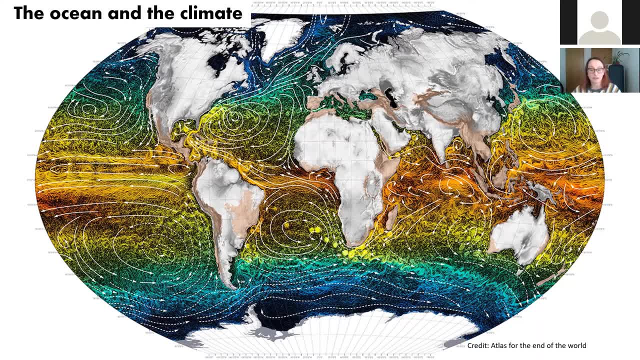 So we can then go study them and extract that information from them. Just as we use historical archives or archeological archives to learn about ancient civilizations, we use marine archives to learn about the past ocean. So when I talk about corals, most people imagine tropical reefs. 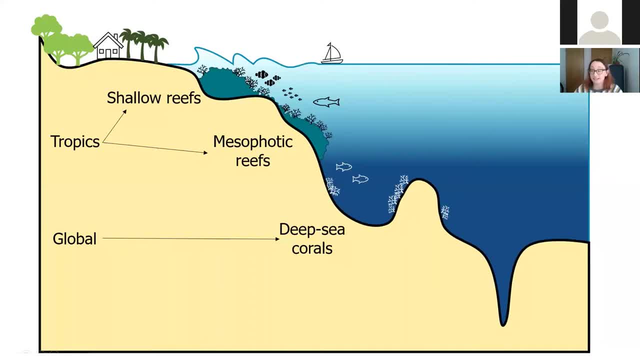 with pristine waters and white sands. And yes, those reefs are built by massive corals that we use as archives. But these corals need very specific temperature and light conditions to survive, And that's why we only find them in tropical regions and shallow waters. 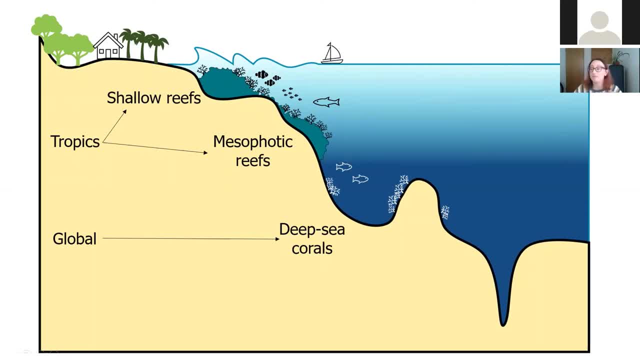 However, they are not the only type of corals. If we go down deeper into the water column, we are gonna find corals down to three 4,000 meters and way below that. They are known as deep-sea corals. 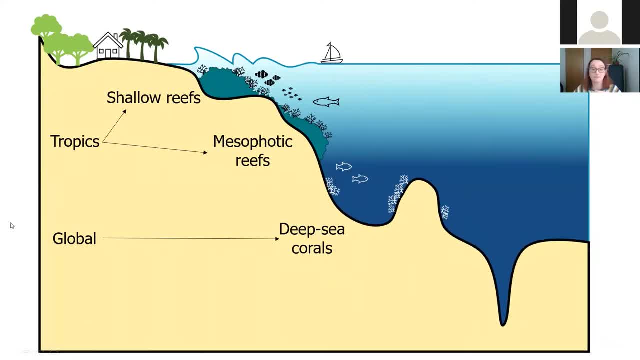 and they don't need sunlight to survive and they can tolerate very cold waters. For this reason, these type of corals can be found all over the planet, from pole to pole. So we have different type of corals in different type of regions and we will study one or another. 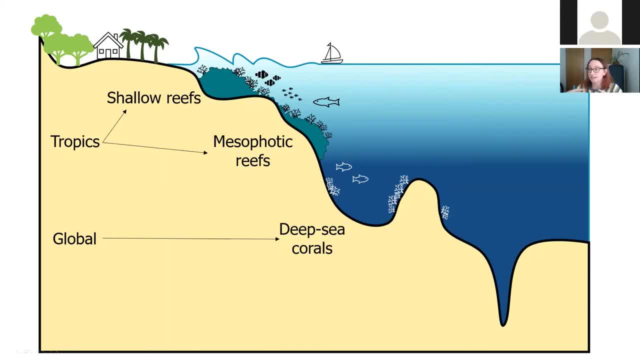 depending on what we wanna find out about the past ocean. They are just like pieces of a big jigsaw that is the past ocean. So how do we do that? We find out what we wanna ask ourselves about the past ocean and we need to go. 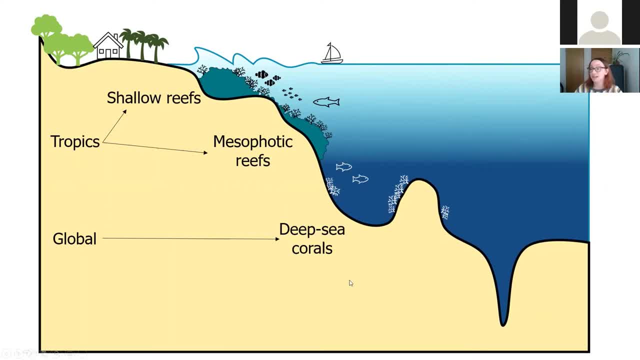 and collect the corals. So, for example, let's say we want to study what was the deep ocean circulation 10,000 years ago To be able to find out that we will need to go into the deep ocean. that would be deep-sea corals. 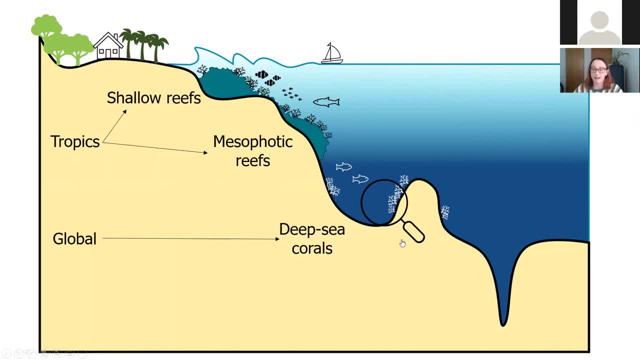 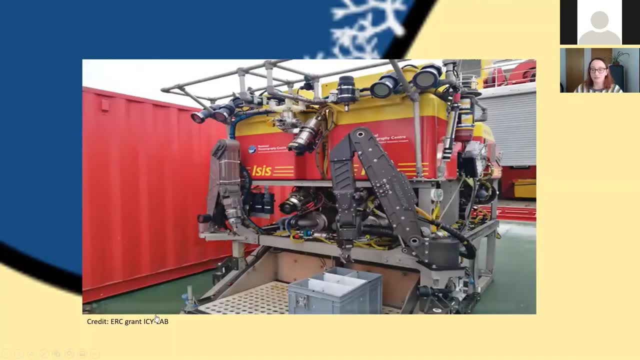 and find out corals that were alive 10,000 years ago. How do we do that? Well, I'm gonna show you. For that, we need RVs or auto submersibles or some sort of vehicle that allows to go deep into the sea. 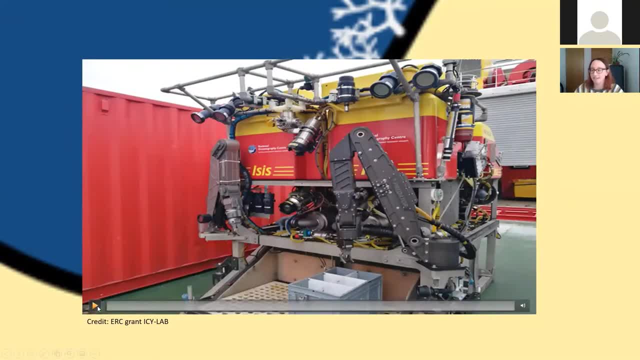 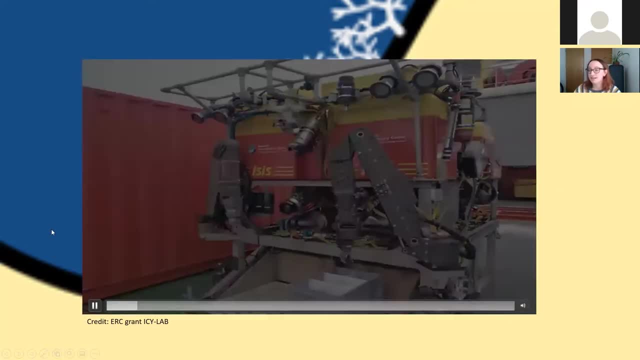 That's because they are so deep down that we cannot dive ourselves. So this one over here, you can see it has some cameras, some arms And then some boxes in here. So we put everything on a ship and we go into the middle of the ocean. 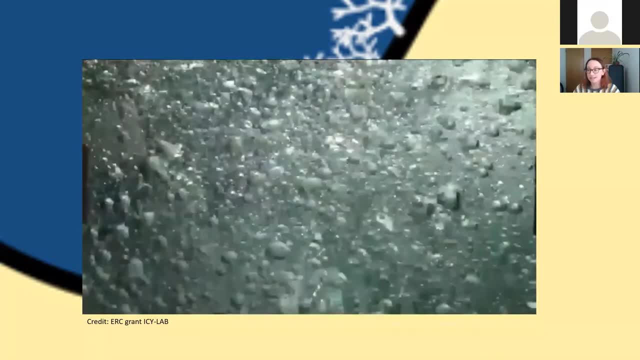 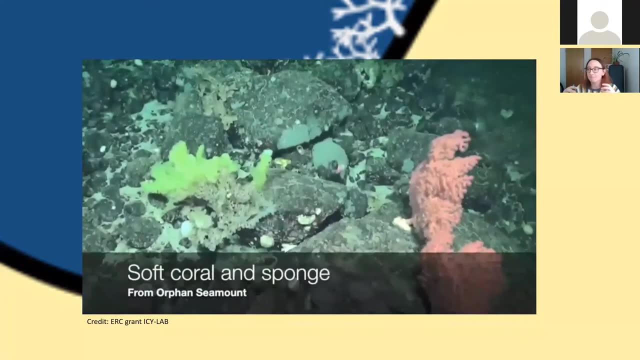 When we are in an area that we are interested in, we just deploy it And eventually it will reach the ocean floor. It is connected to the ship and we are from the ship driving it. So we get there and we find what is the ocean floor like. 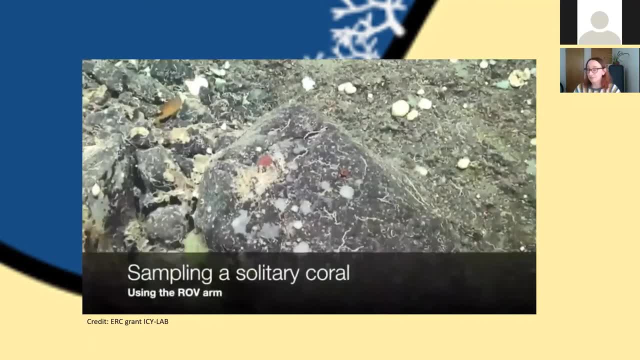 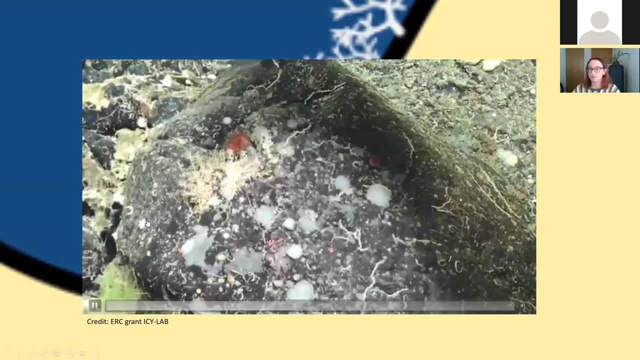 And we start looking for corals. Once we find the corals, we want to, we need to collect them, And that's what we can see here. We found one coral over that rock. We want that coral to study it. So then we take the robotic arms. 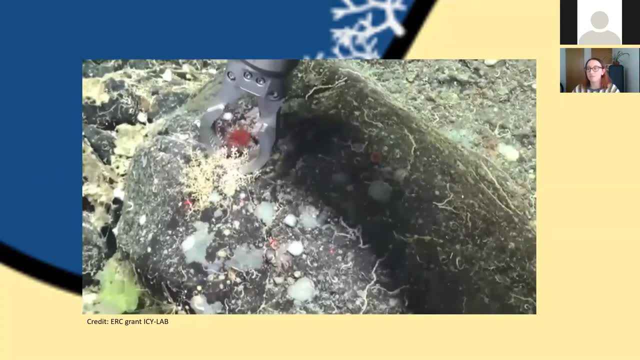 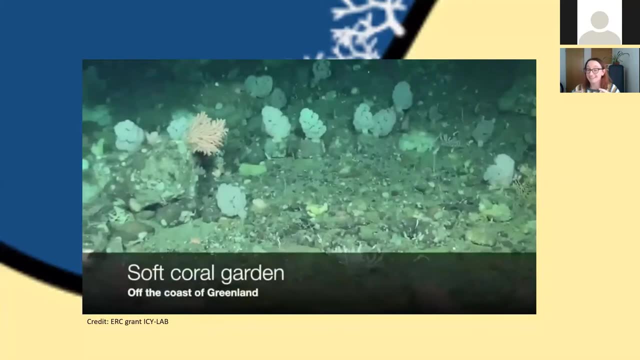 and just like a video game. with a joystick, you pick up that coral and put it in a box and keep looking for more corals. So it's a high-precision job, but it is extremely cool. Deep sea corals don't form reefs. 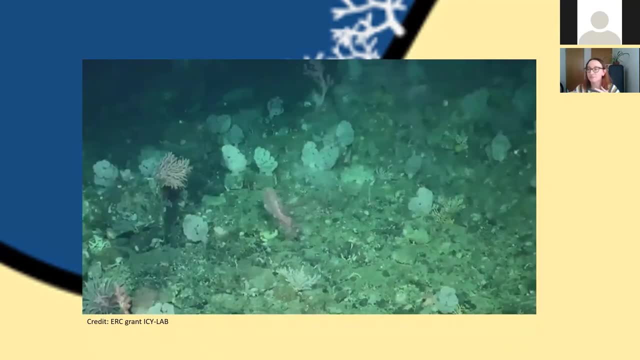 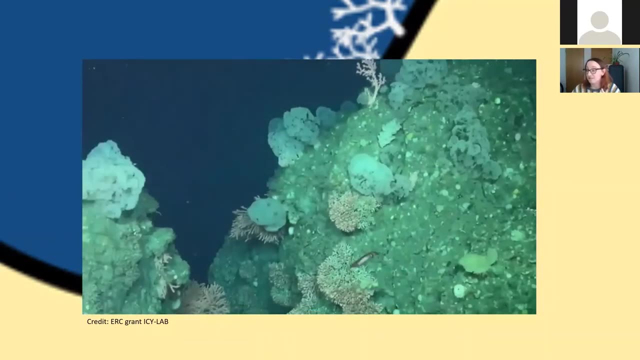 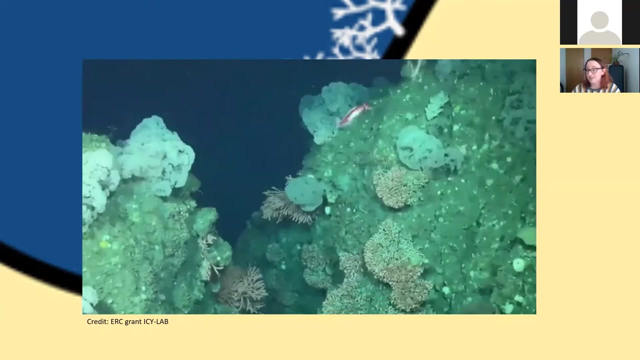 as the reefs that you are used to see in tropical regions. They form coral gardens, but they are still extremely beautiful and chances are you are the first human being that are seeing that piece of ocean floor when you are there, So it is proper ocean exploration. 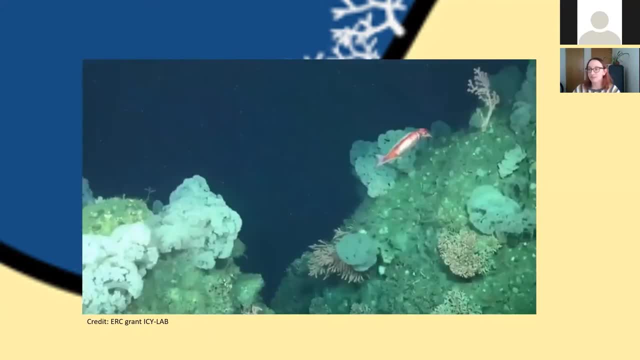 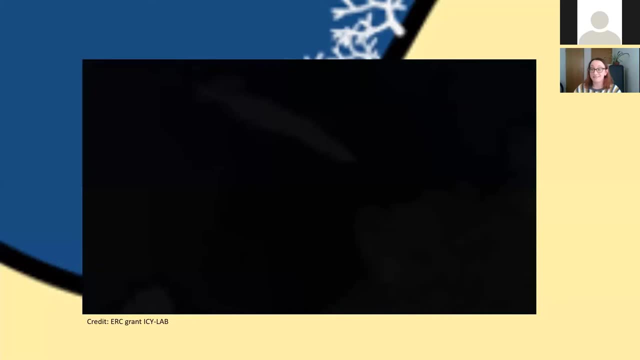 And I think it's one of the coolest thing I have ever done. This footage is from an expedition we did with the ICELAB project on the Labrador Sea west of Greenland, And it was just very, very cool, Excellent. So that's for deep sea. 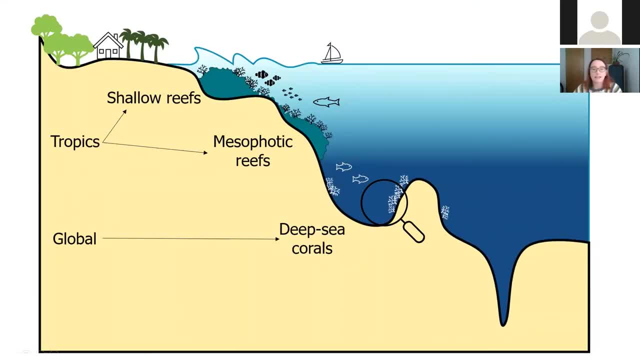 If we wanted to study, for example, what you know was the variability of the monsoon 500 years ago or a thousand years ago, then we would need to go and study shallow tropical reefs And we would need to get there and collect some of the corals. 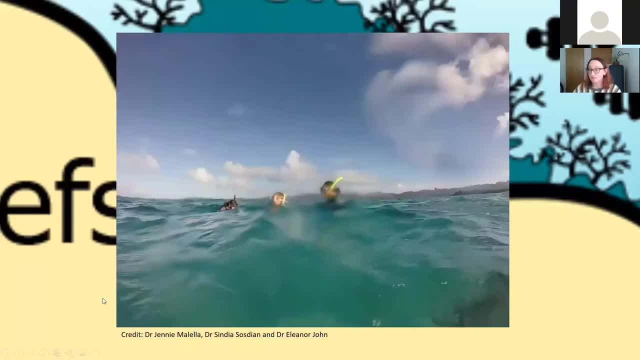 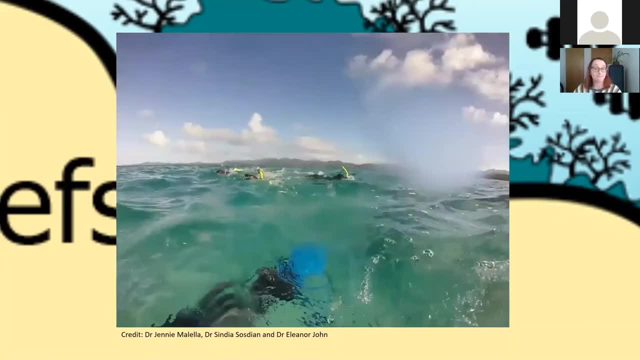 How do we do that? Well, we literally need to jump into the water. This is some footage on an expedition in Fiji from Cindy Sosyan and Eleanor John. They are my supervisors at Cardiff University. So you go there, you put on your scuba gear. 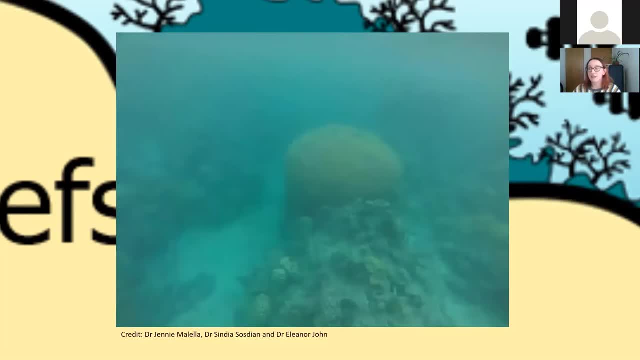 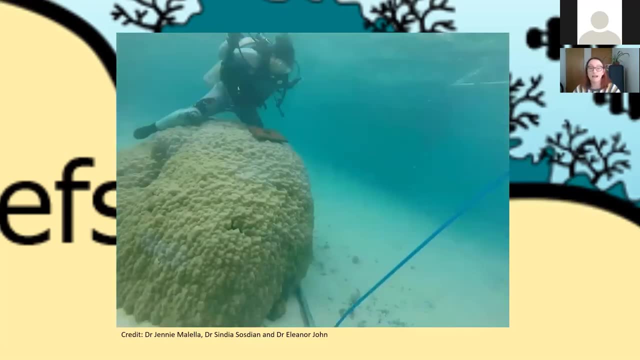 and you find a coral head that is big enough and healthy enough. And because they are very big, we cannot take the whole coral back to the lab with us, So what we have to do is just take a piece of it. We literally drill a cylinder of coral material. 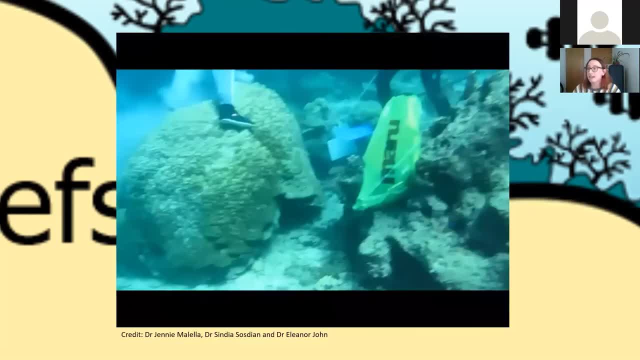 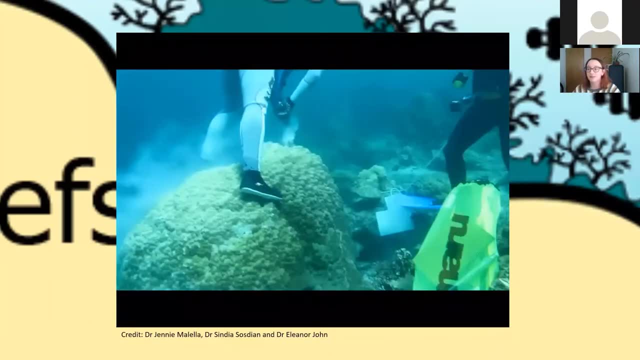 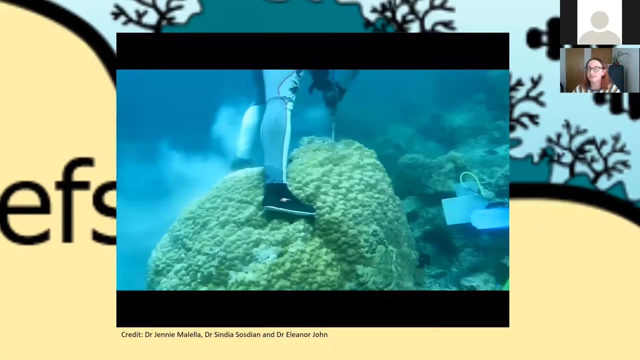 is what we can see there And that's the piece that we take with us. So this in this is footage. with a pneumatic drill, We take a cylinder called coral core And then the coral head remains on the reef And we take our piece of coral with us to the lab. 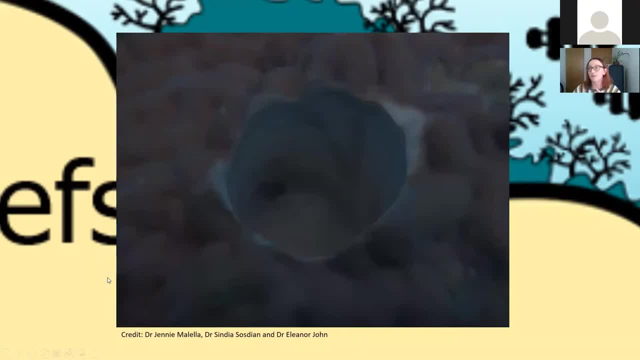 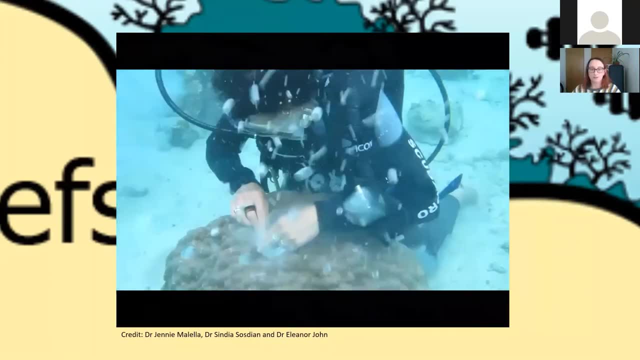 That's the coral core that we take with us And that's the hole that we leave on the coral head, And then we need to make sure that we cover it with a cement block, just so other organisms don't get inside the coral and get infected. 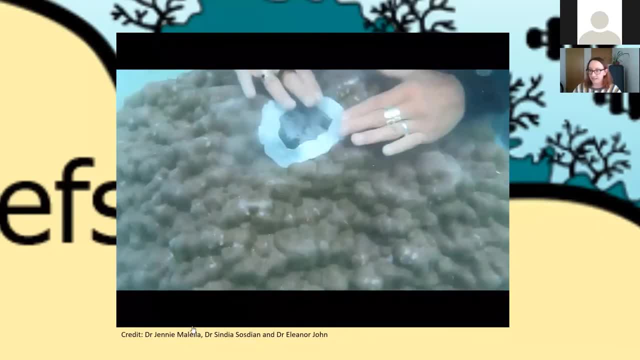 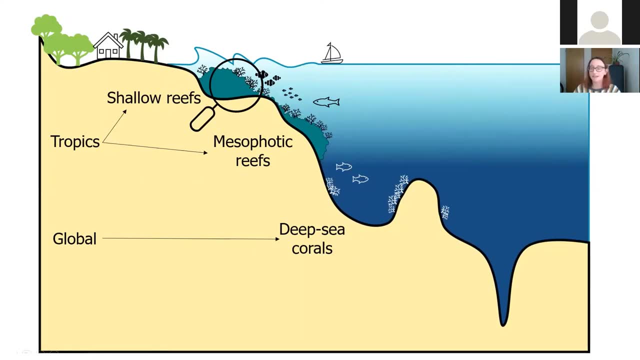 and transmit some disease, Right. so where were we? We decided that there was a question about the past ocean. We wanted to ask whether it was deep ocean circulation or was tropical climate in tropical regions. We went there, we collected our corals. 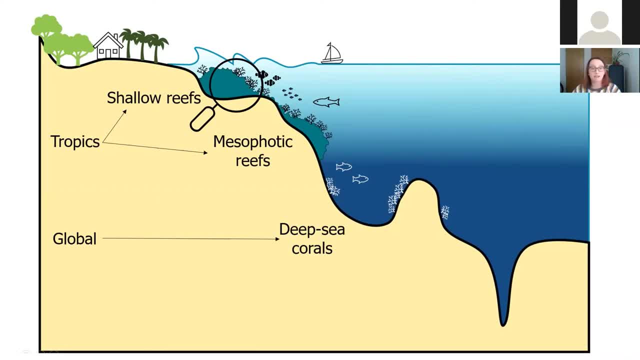 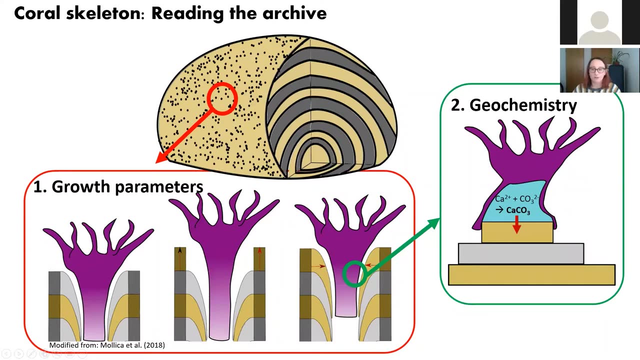 We have our corals now in the lab with us. How do we extract the information We are interested in? how do we read these corals that we collected? Right so, deep sea corals and tropical corals, or shallow water corals- they are somewhat similar. 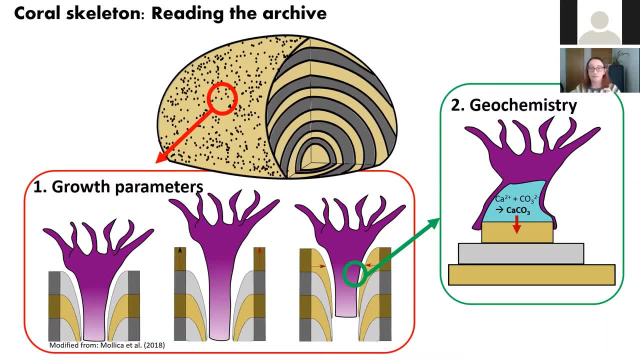 in terms that they both build a skeleton out of calcium carbonate. It can be calcite or aragonite, depending on the species, And it is basically limestone. They build a rocky, stony skeleton- The information that we are after about the past ocean. 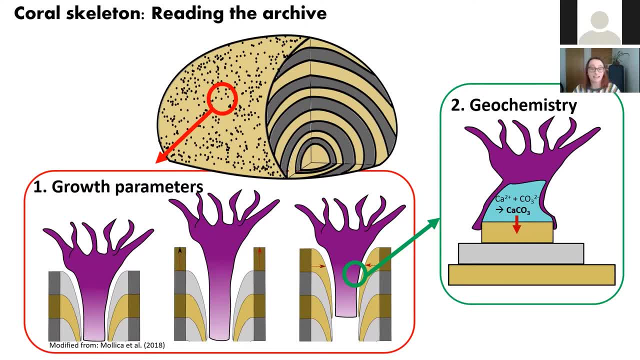 is within this skeletal material. We are interested in the skeleton of the corals. And why can't we find environmental information in the skeleton? How is it that corals can record that environmental information in which they grow in their skeleton? Well, that's because some corals, as they grow. 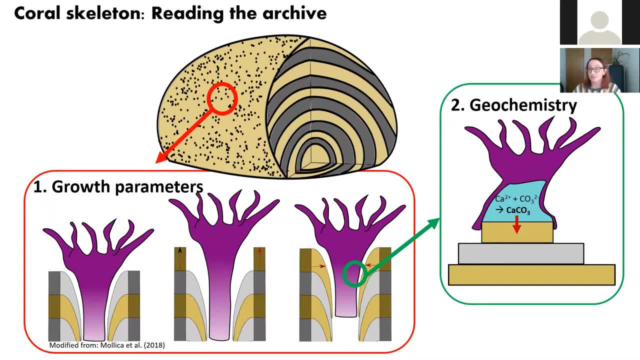 they grow in bands, just like tree rings, And just as we can extract some climatic information from the tree rings, we can extract some environmental information from the skeleton of the corals as well. So that's what we see here. The purple bit is the poly. 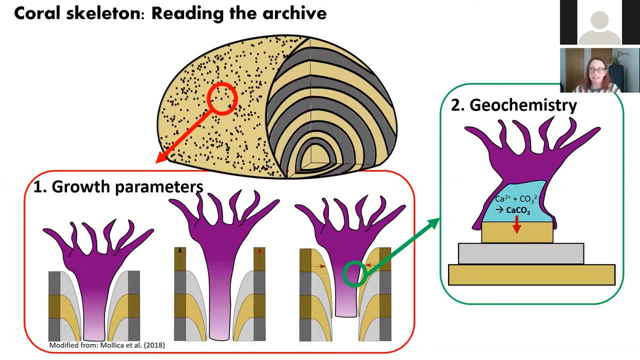 is the leaf, The living part of the coral, is pretty much like a jellyfish: has some tentacles and just for defense and feeding, And every season or every year, as they grow upwards, they build a new layer of the skeleton. 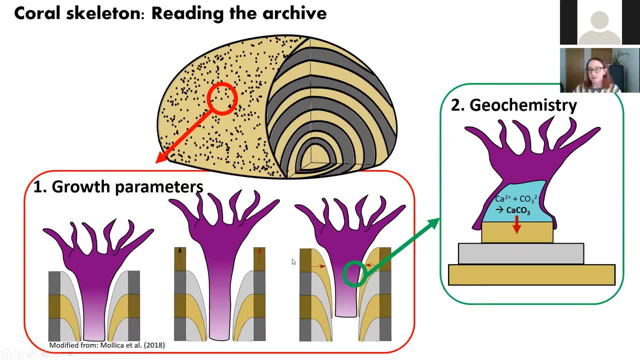 This layer of the skeleton will be larger or shorter, or more dense or less dense, depending on the environmental conditions. Let's say, for example, one year is warmer than usual, The coral might grow faster, and then we'll have bigger band and less dense. 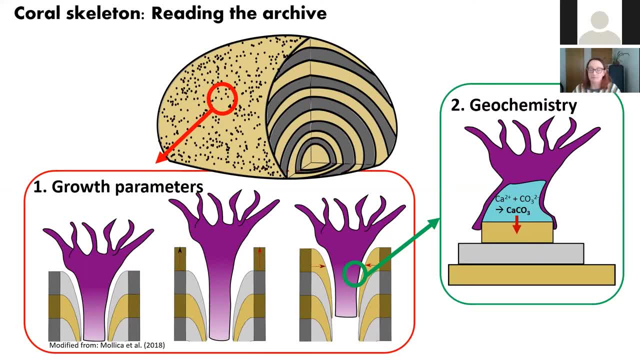 But if it's too hot it might stop growing whatsoever and will have no growth or a very thin and very high density growth. It depends. That's how we can read the physical properties of a coral skeleton. And if we go one step further, 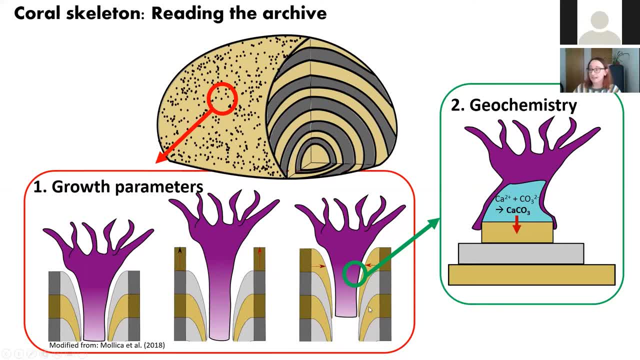 we not only look at the physical characteristic of the skeleton, but we look at the chemical composition of this rocky material because, for example, this is a very, very small coral. So this is a very small coral that builds their skeleton out of seawater. 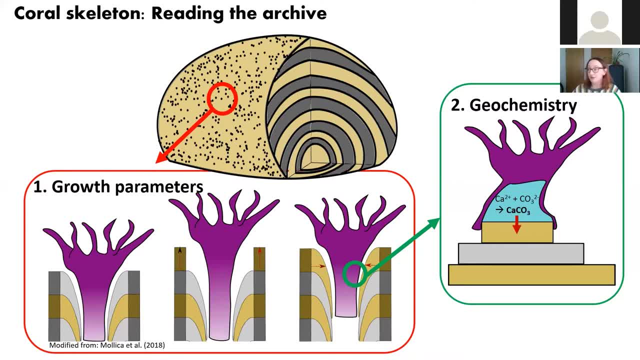 They get chemical elements from seawater- might be calcium and carbonate that is dissolved- and they combine them to form this mineral called aragonite or calcite, And along with these elements, they also introduce different elements like strontium or barium. 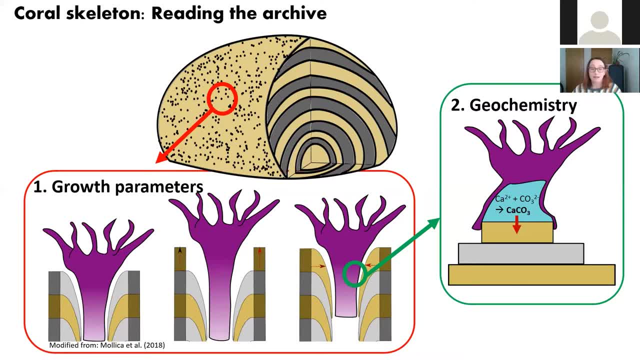 And we can measure how much of these elements are there in the skeleton And then we can understand what we can do. What's the temperature back in time? If there is more or less strontium, that means that the temperature would be higher or lower. 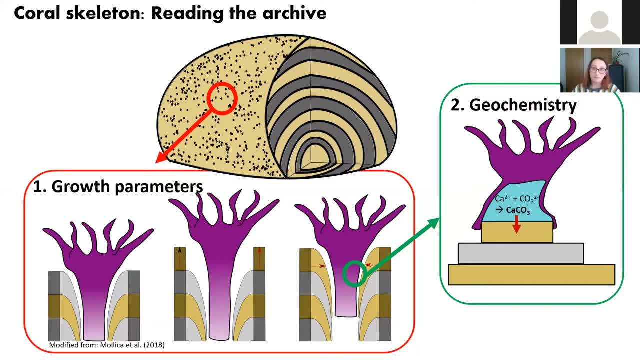 Or if we have more or less boron isotopes, we can guess what was the pH or the alkalinity of the water. We can measure, I don't know. carbon or nitrogen isotopes more or less would tell us if the productivity. 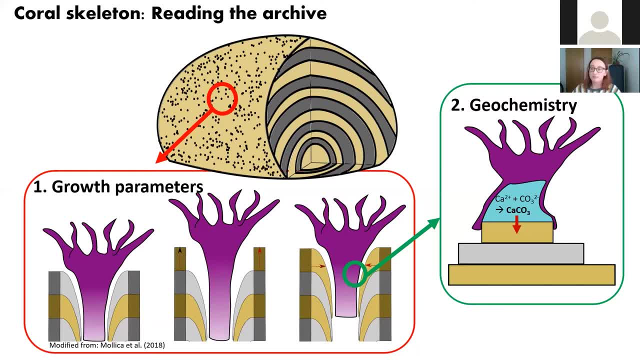 was higher or lower, if there was a lot of nutrients in the water or if there were no nutrients pollutants. There's a range of environments and environmental information that is within these coral's skeletons And how much information of how far, how deep in time, can we go with corals? 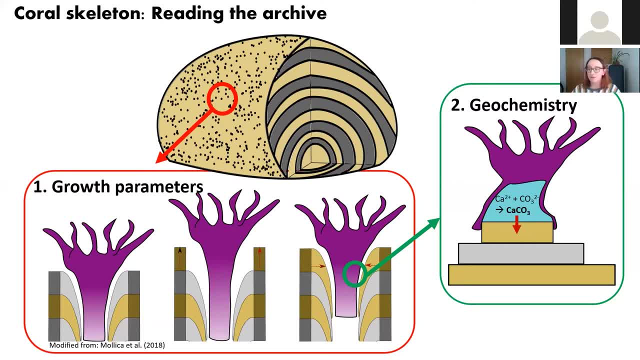 Well, that's going to depend as well. Most corals have a lifespan of a hundred years. However, some deep sea corals have been found to be able to live up for three 4,000 years, which is, it's, mind blowing. 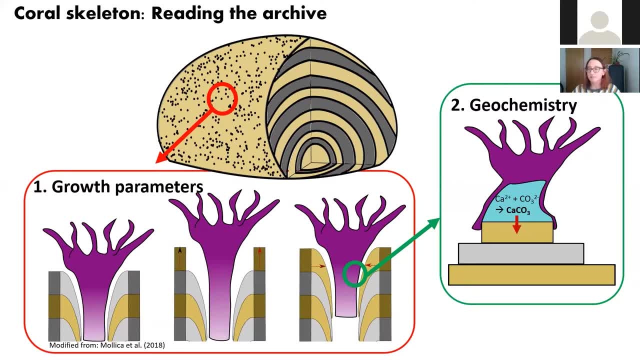 But that means that with one single coral we're going to be able to measure lots of environmental information from hundreds and hundreds of years. That means that if we get a coral, collect a coral that was alive today and has lived for 500 years. 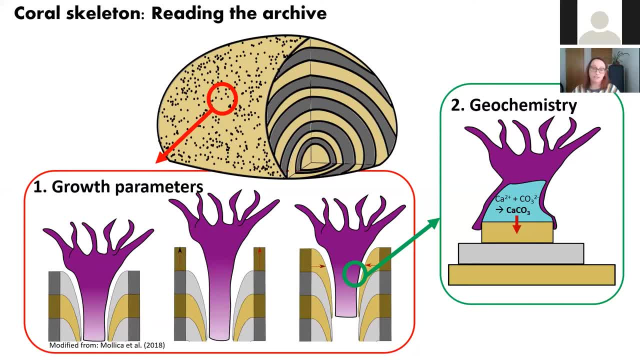 we can measure ocean temperature, ocean salinity, nutrients up to 500 years back in time. But because this information is within their stony skeleton, is within their skeleton. once they die, they get preserved as fossils And they get preserved for thousands and thousands of years. 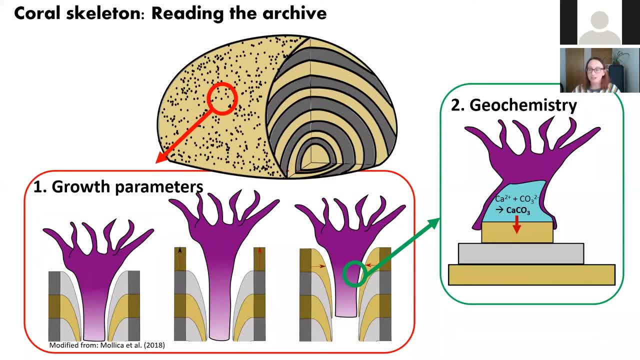 So we are able to reconstruct environmental conditions up to a hundred years- sorry, a hundred thousand years- in the past, which is enormous amount of time, And it is extraordinary. And, yeah, corals, they are just extraordinary. So how do we extract this information? 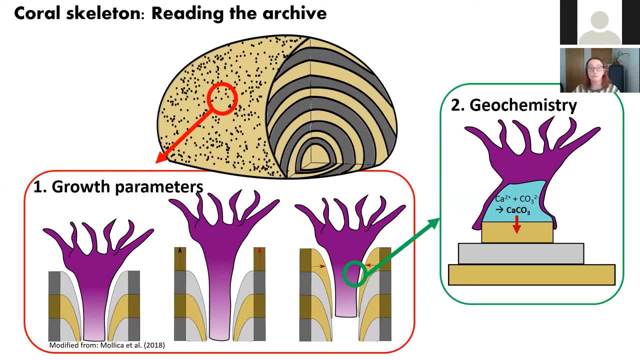 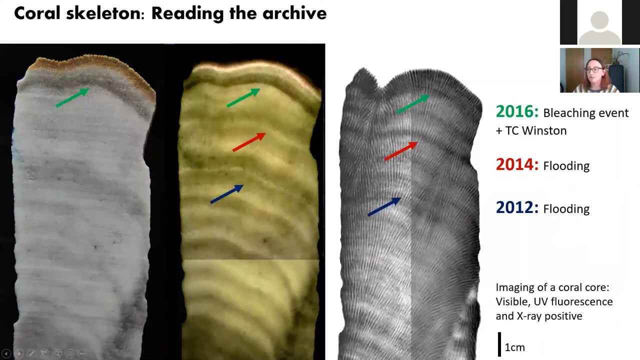 We know they record this information. We know this information. It's in their skeleton. We collected the corals. Now how do we read it? What does it mean? What I have here is three images of one of the coral cores that we show before were collected in Fiji. 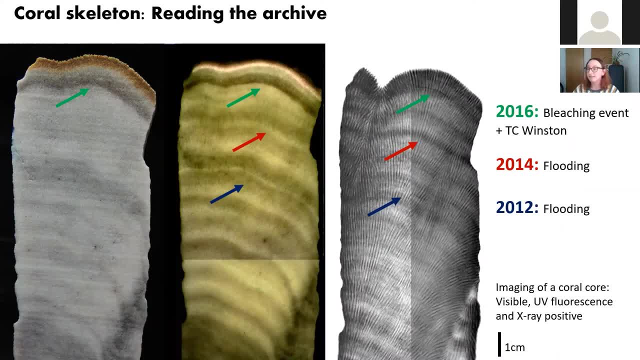 in a tropical reef And it's just the core split, half in open, And it's a picture under normal light, a picture under UV light and an X-ray from CT scans, like the ones you get when you go to the hospital. 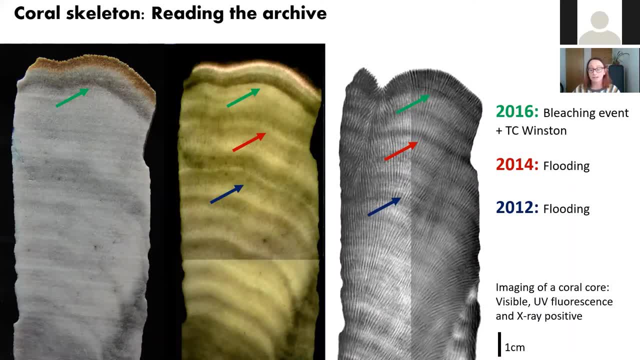 Well, we can see is that the growth bands, the growth bands that we were talking, before they become visible, And because we can see them, we can just count down from the time where the coral was collected. So this one in particular, collected in 2017,. 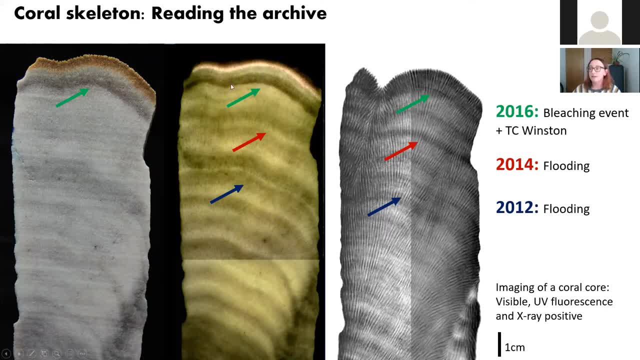 we can count. one year below is the band below. We see a very dark area here, high density area here. So we can ask ourselves: that's 2016,. one year below. What happened then? Well, in Fiji happened to be. 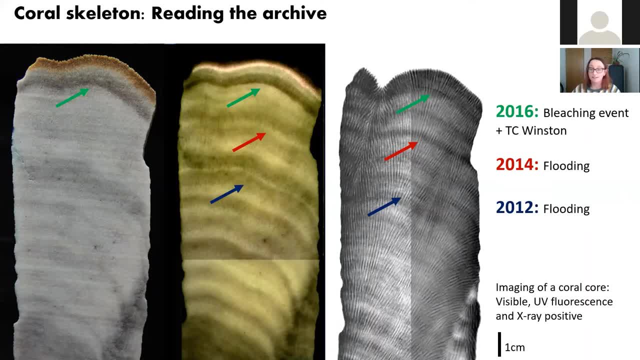 there was a bleaching event and there was a very strong tropical cyclone named Winston, which caused several damage on the islands, several flooding, and that can be reflected on the coral skeleton And like that we can go down hundreds and hundreds of years. 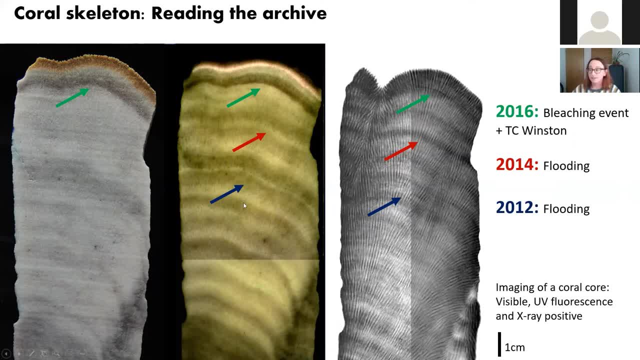 Once we know what year correspond one section of the skeleton like, for example, we count down and we know that this area here corresponds to 2012,, we can collect a bit of that skeleton, put it on a mass spectrometer, which are machines that are so extremely sensitive. 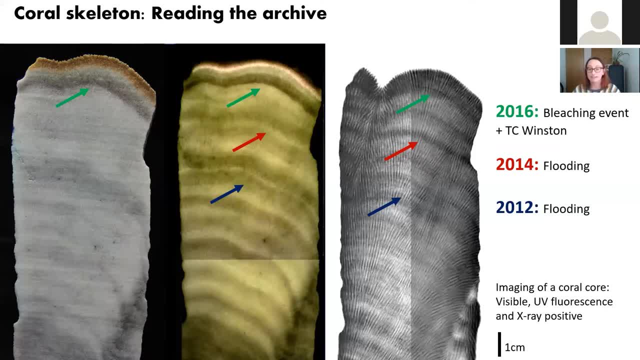 they can measure very, very small amounts of different elements And we can extract information from, as we were saying before, barium, strontium, lithium, boron, carbon isotopes, oxygen isotopes, and that will give us information. 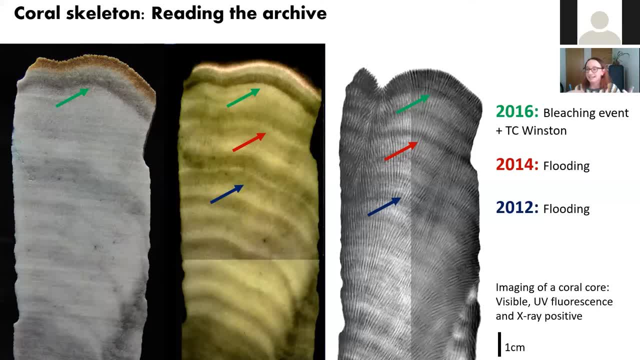 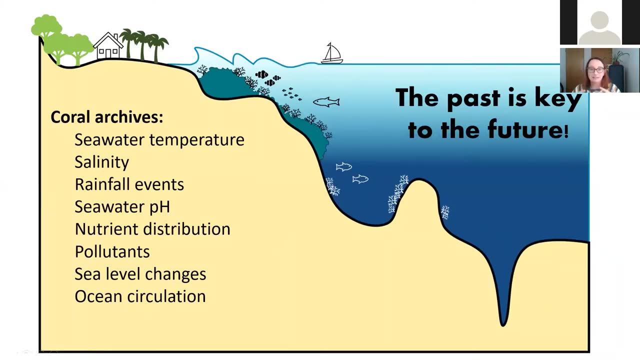 on temperature, salinity, pH, sea level changes, ocean circulation and that whole wealth of information Just from one single piece of coral. So just to resume, the past is key to the future If we want to understand the climate. 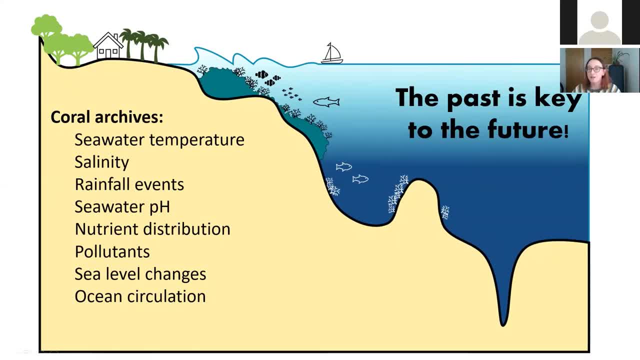 if we want to predict what the future climate is gonna look like, we need to understand the past, And corals contains information on past ocean temperatures, salinity, nutrient distribution, pollutants, sea level, et cetera. They're incredibly valuable for paleoclimate scientists. 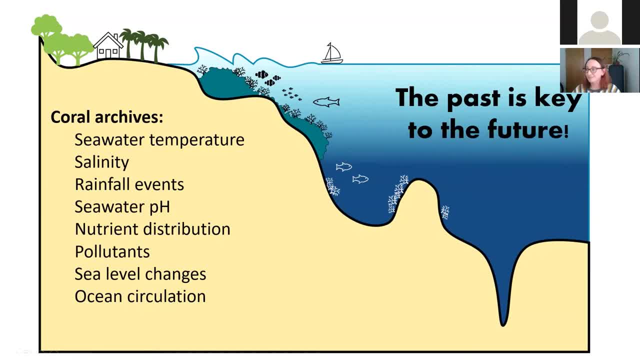 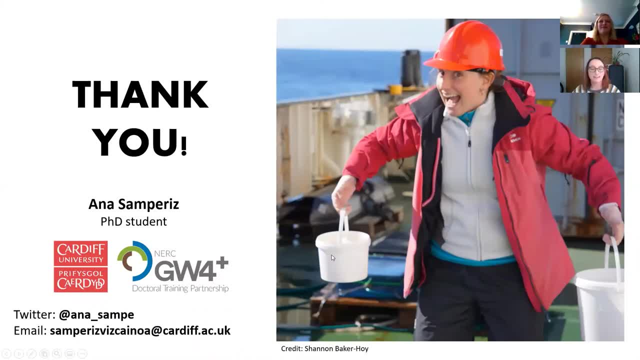 and that's why we're studying them. And that's all from me. Thank you very much. If you would like to know something else, I have my contact details. Just drop me a message and I will more happy to pass you on more resources. 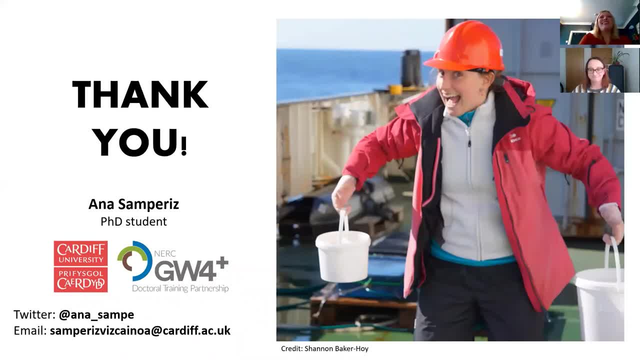 or more information. Thank you so much. Thank you One question already, and that's actually about: do submarine volcanoes affect any sort of coral reefs And is there any way to possibly reach out to them? that's actually about: do submarine volcanoes affect any sort of coral reefs And is there any way to possibly reach out to them? 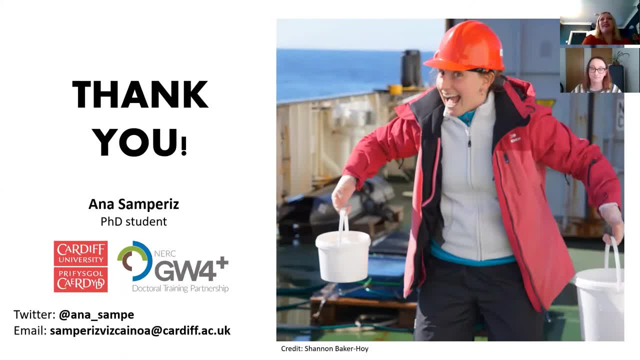 construct gases emitted or understand the history of eruptions underwater? Yeah, most definitely. Whatever is going on in the environment surrounding this coral is going to be reflected. Submarine volcanoes might change the temperature of the water, might change the alkalinity of the water. 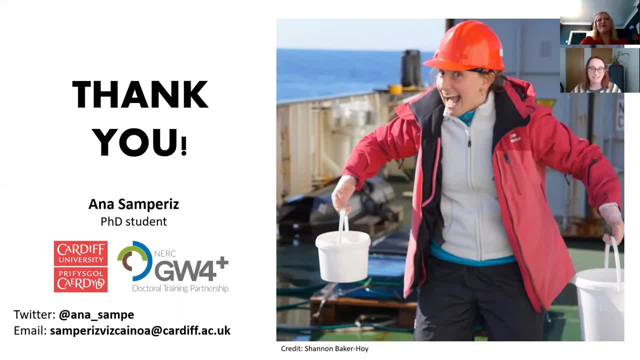 and that's going to be reflected And we can measure that and we can time when there has been volcanic eruptions, whether they're submarine or not. All this type of information is contained within the corals. Excellent Thanks, I think. hopefully we'll get a few more questions in. 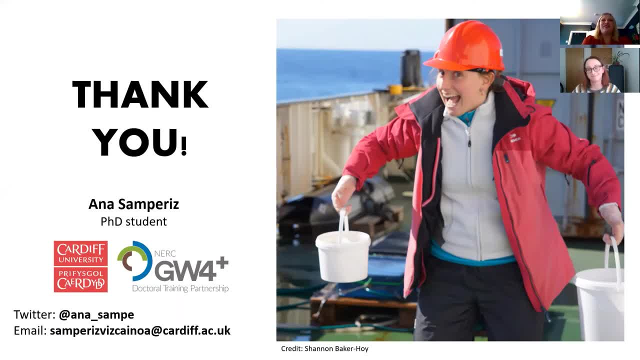 But my question is: what attracted you to this field And why did you choose to go into geology as a degree? That's a very good question. I'm not sure I have a clear answer to that. I guess that I've always been very curious about. 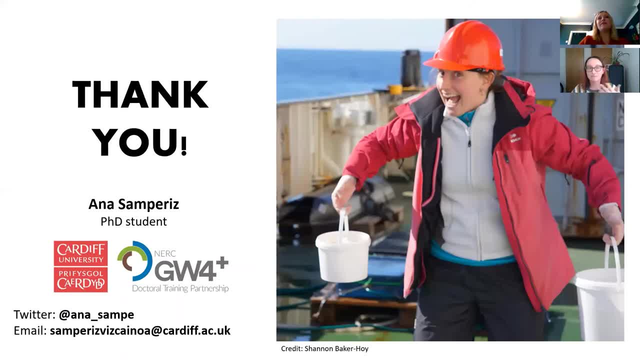 the environment, about nature, about different processes happening, And I guess once I knew I wanted to go to university and do a Florida degree, I did environmental sciences but I wasn't sure I wanted to do environmental sciences or geography or geology. 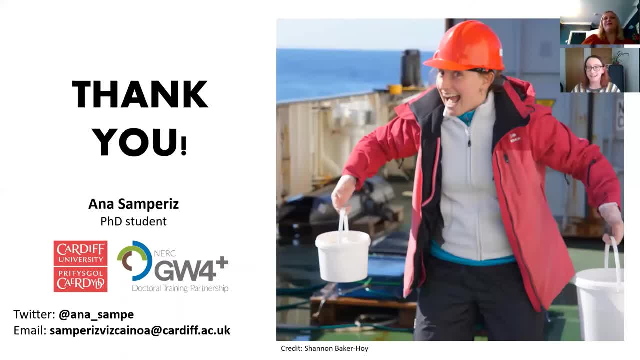 So I just wanted to know more about the environment, and that's what drove me, Great Thanks. So you've got another question and that's what is the most interesting or unexpected thing you've learned about the past? Ooh, that is a difficult question. 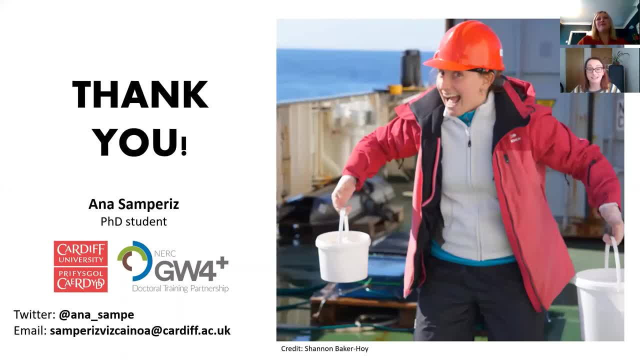 I'm not sure it would be the most interesting- I could say definitely unexpected- for me would be that when I started working on Fijian corals, well, I was just kind of expecting the corals to be decreasing. They're resilient. They're resilient because, on the last 100 years, seawater temperature has been constantly increasing And what I found is that most Fijian corals were very happily with this temperature increasing and they were just growing faster and faster, which is good news. 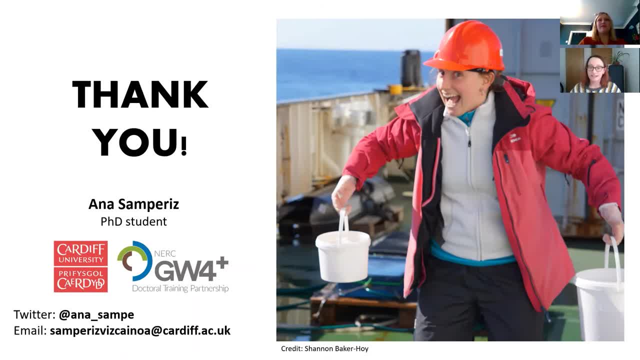 However, that's not widespread. That's not always the case. It really is very site-specific, But yeah, it's something I was not expecting Great. Is it possible to identify events recorded in the coral that are global rather than regional? 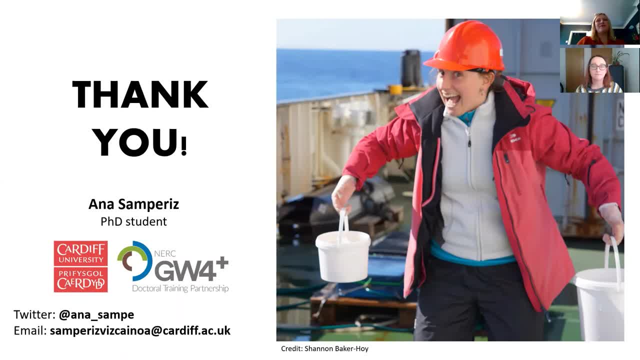 Most definitely Something comes to mind. For example, lots of people use these corals to study El Niño Southern Oscillation. That's a climatic global event that's like in the Pacific Ocean and in the atmosphere over the Pacific Ocean. 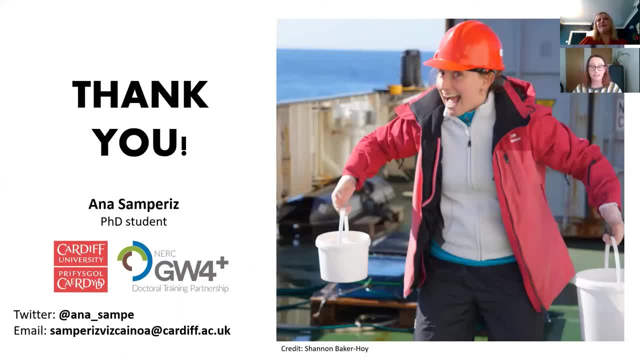 The currents just change. Change, Change in strength, Change in direction. Everything changes in order, And it affects both Asia, South America, North America. So, yeah, that's a global event And that can be recorded on the corals. 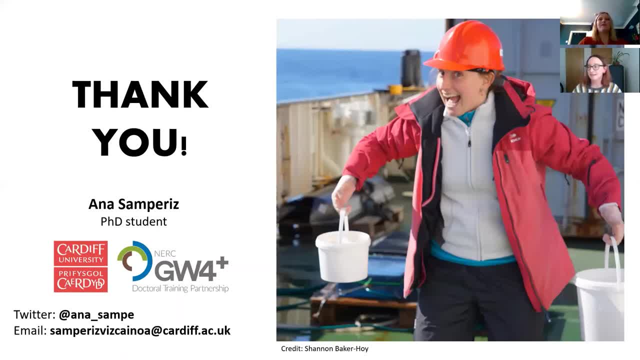 So obviously, corals are very regional, But there are some changes that, although they can be detected regionally, that is a global change And we just need to learn from different pieces from different regions to understand how, how regional effects are part of a global effect. 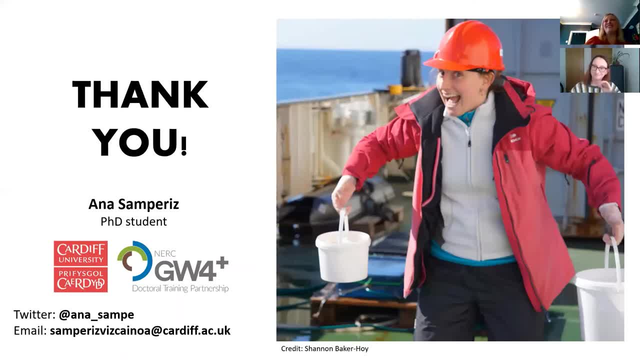 if that makes sense, Yeah, that's great. Thanks so much, So we still have time for a few more questions, if anyone wants to post them. I guess for me it's: what do you enjoy most about the work you're doing right now? 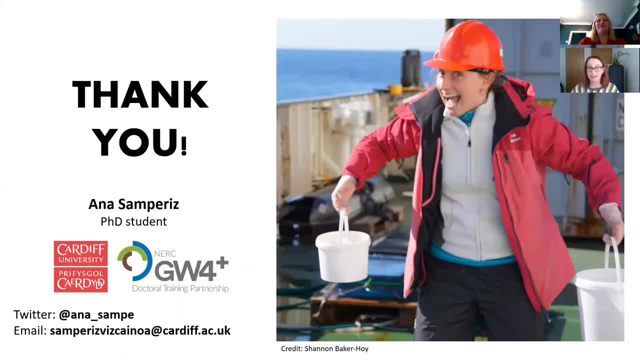 I think that my favorite part is always the field work. I just really like field work. I love going out, getting into the field and collecting the corals, Seeing them. It's just a very cool feeling, So that's one thing that I really enjoy. 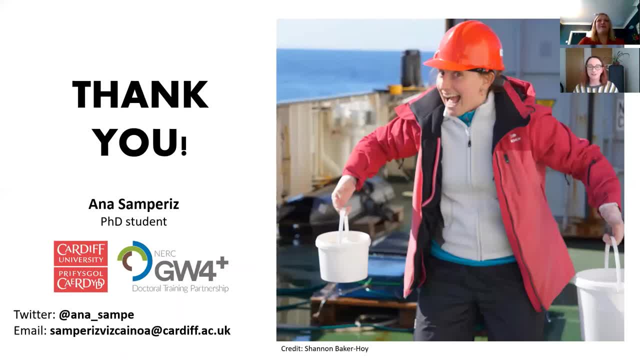 But besides that, I really, really enjoy that part when you first get a batch of data after analyzing your corals And you are the first person ever in seeing that data And you are the first person ever in trying to find out what's going on with that coral. 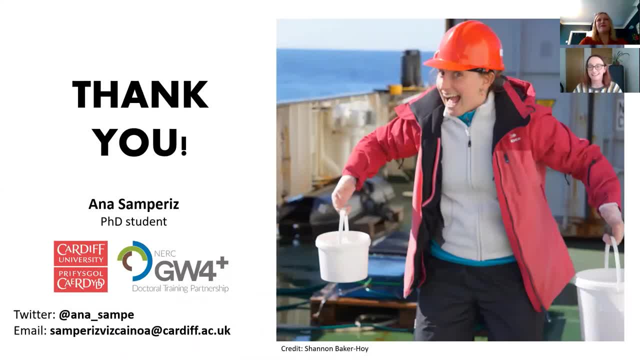 and what it means and what is going on, And that's a very cool feeling. Maybe it's because I'm a nerd And I like science and corals, But being able to see the data for the very first time, it is a very good feeling. Great, So I've got now. do you find the same species of coral now and in the fossil record? Yes and no. It depends how deep we go in the fossil record. If we go from a few thousand years back, 10,, 20,, 30,000 years. 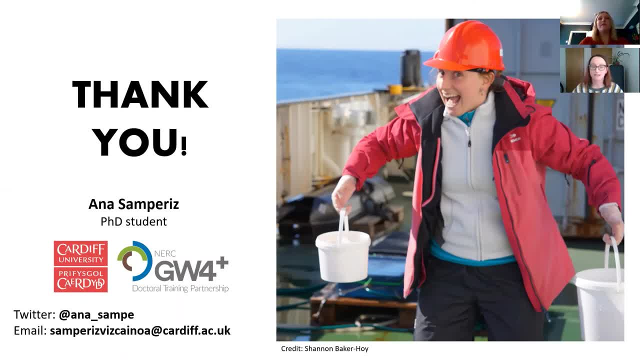 back, we have similar species. If we go further, deep down in time, they are somewhat different. But although they are different species, they are very similar to what we have today And in a sense they all build as carbonated skeleton, which 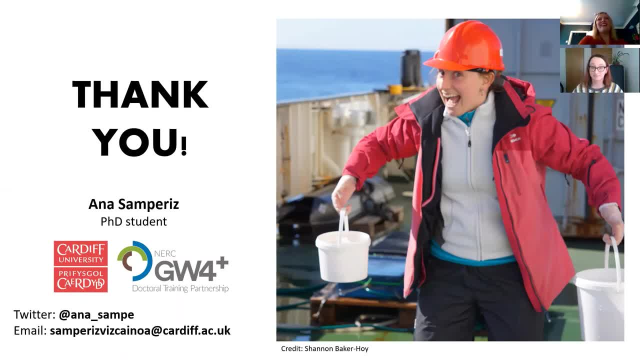 is what we are interested in. Great, And this is about why did you move away from working solely, I guess, in this environmental element of the environmental science? Ooh, Yeah, Yeah, Yeah, Yeah. Difficult, I guess, because I like to do research. 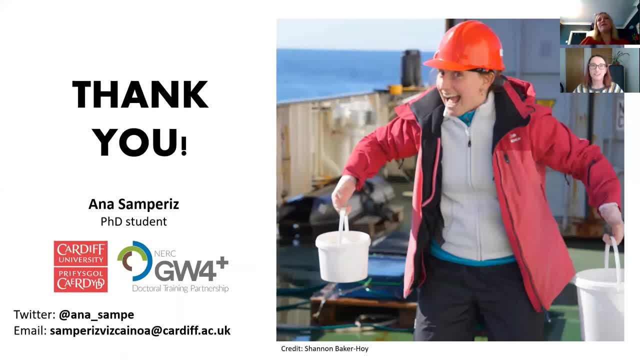 And when you get into research, you need to specialize in a very niche, in a very concrete thing. It is hard to do research in a multidisciplinary area, being able to cover a lot of topics. You're focused on one. You collaborate with people with different areas. 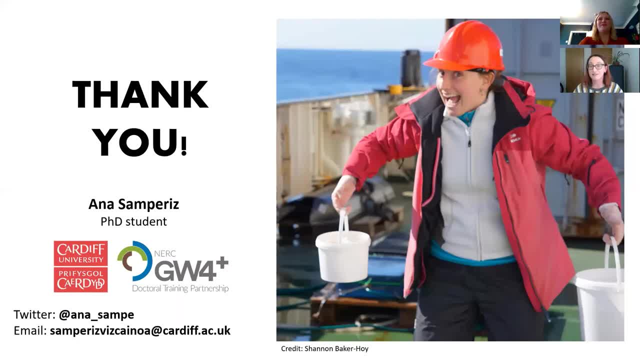 and that's what makes a good science. But when doing research Mostly, and me personally- it is so hard. You need to focus in one topic, in one thing and go for it. Great, And here's a good question. 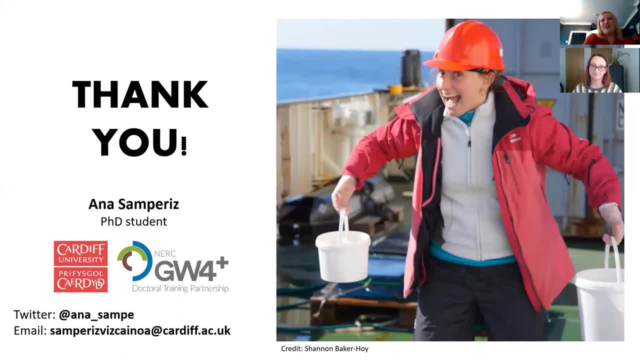 So I absolutely love biology and geography, but I'm worried I have to drop one for the other. How much does geology and biology overlap within your degree Right? Well, because I did environmental science, I think, or at least the program I did in my university. 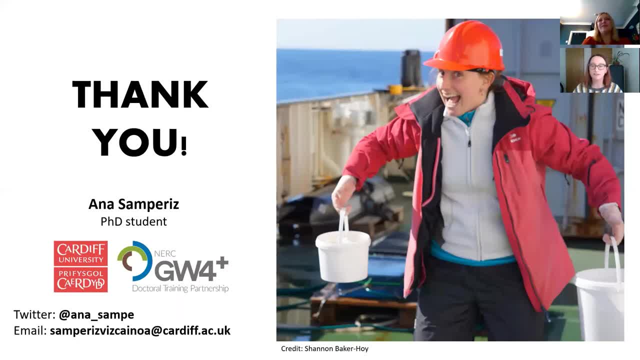 it was a bit of jack of all trades. We had a bit of geology, We had a bit of biology, a bit of ecology, a bit of economy. So it was a multidisciplinary program. I think that, if you like both you, 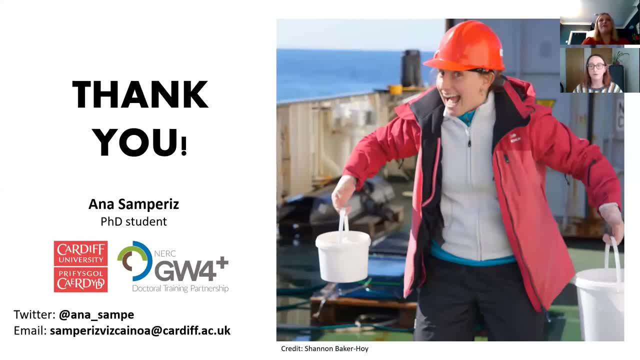 can find programs that have bits of both. You don't have to go into one or another, And even if you go from one to another and then further, you want to change to a somewhat different field. If you start biology but then want 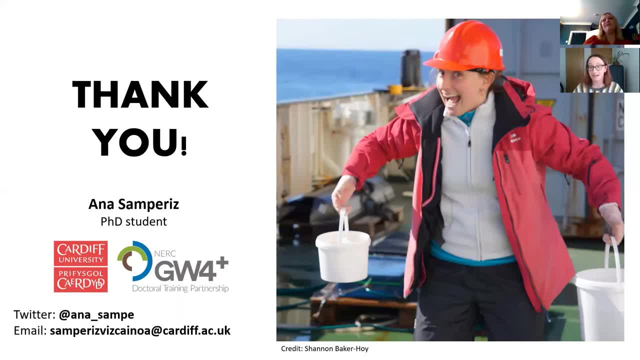 to go into earth sciences or geology. it can be done because the field is so multidisciplinary that although you choose one doesn't mean that you're going to end up in that field forever. You can jump from one to another And the knowledge you learn you're. 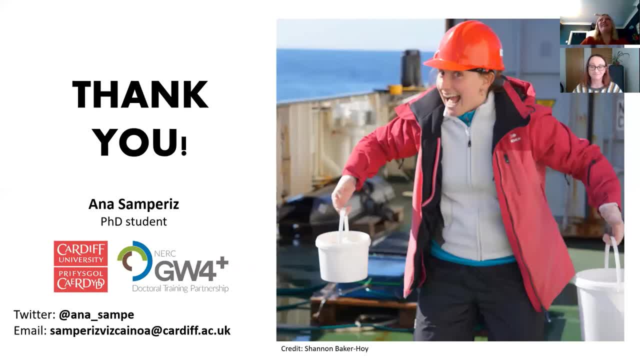 going to have that with you. Yeah, Maybe I can add a little from my experience. I did something similar where I did a geology degree but then ended up studying fossils as well. And yeah, I like to think of earth science as just applied physics. 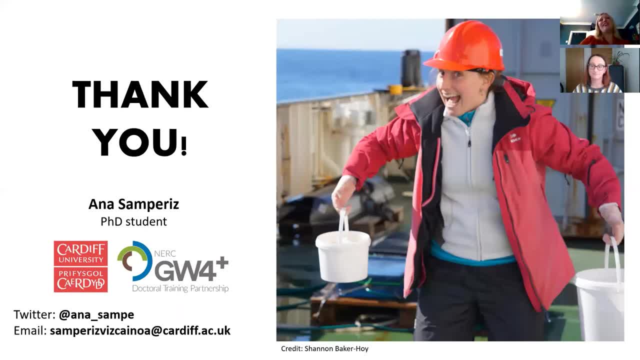 chemistry and biology, in that you're taking that and applying it specifically to the earth. So, yeah, you can overlap many disciplines with geology quite easily. And, as someone else, ooh, this is a tough one. Would you suggest a geography or environmental degree? 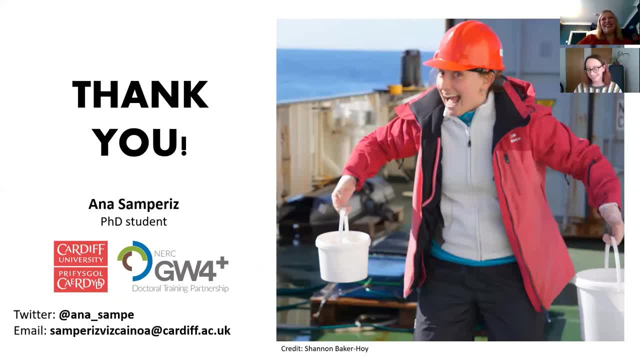 Because I love them both. I love both. Geez, I don't really know myself. I guess I would say environmental degree, because this is what I did. So in my experience I learned a lot, And a lot of things I learned were very useful. But I'm sure a geography program would be equally useful. I think what I recommend is to have a look at those programs in the universities that you want to go and see what they look like, Because sometimes geography that is more from the social and human side or more from the 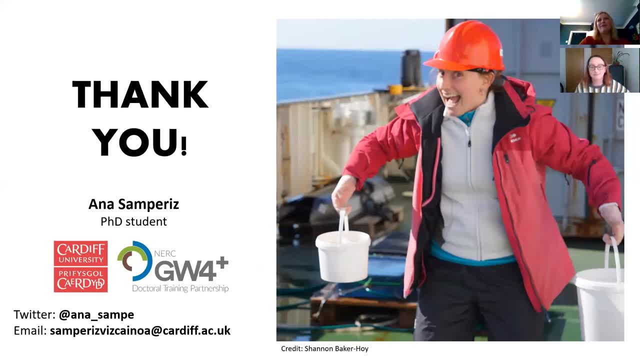 like physical or environmental side. But wow, that's a difficult question. If I had to choose again what to do- geography or environmental science- I would be in the same situation where I don't know what to do. I think the nice thing to you and I'll. 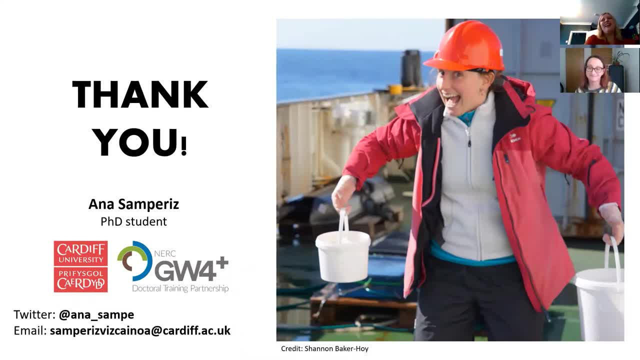 do a little plug here, for the Geological Society's website is you can go and look at our careers pathways finder And I think you'll find that geography and environmental, environmental degrees and geology degrees can lead you to very similar or some of the same jobs. 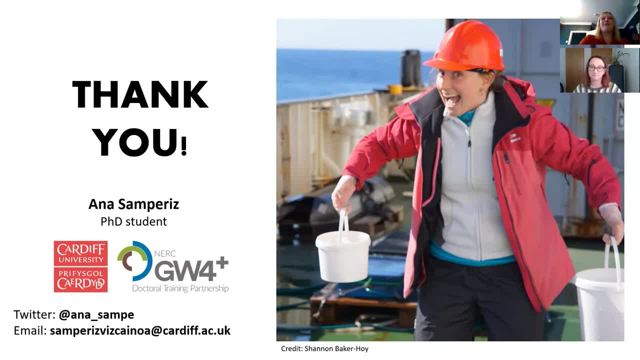 And it just might be slightly different specifications depending how much you want to go down, like an engineering route or a more contaminated land or sustainability route. So definitely check out our website and check out the degrees, And I think we're actually about out of time.